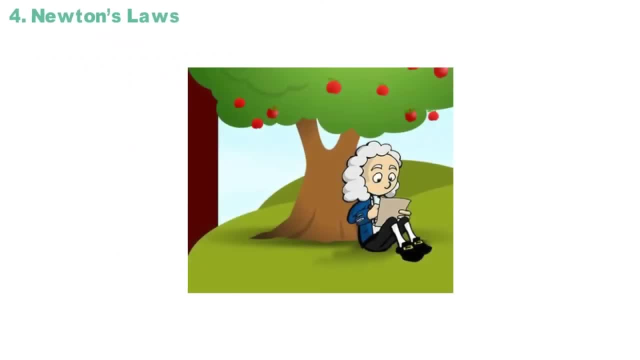 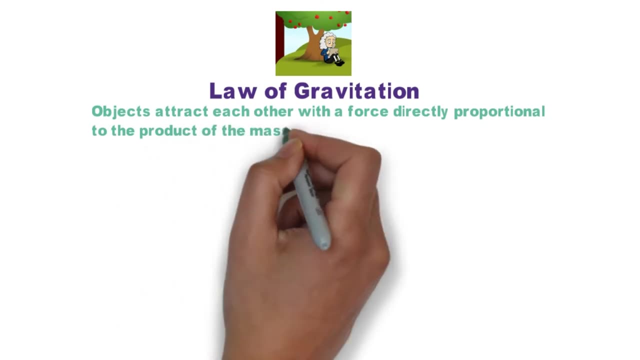 4. Newton's Laws, Law of Gravitation: Objects attract each other with a force directly proportional to the product of the masses of the objects and inversely, proportional to the square of the distance between them. Hence, for objects on or near the Earth, 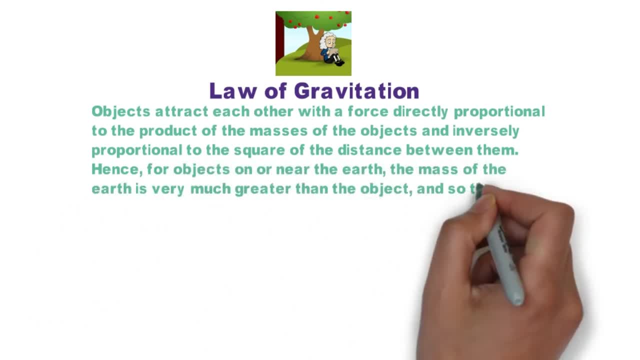 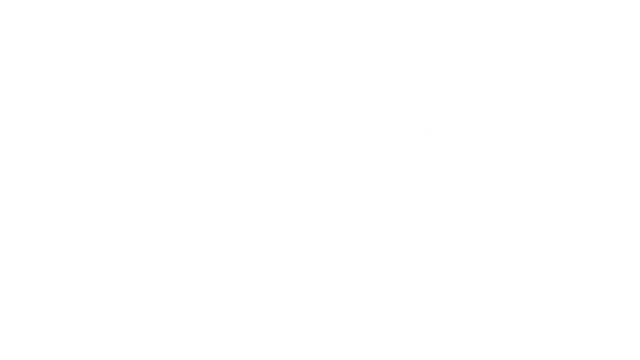 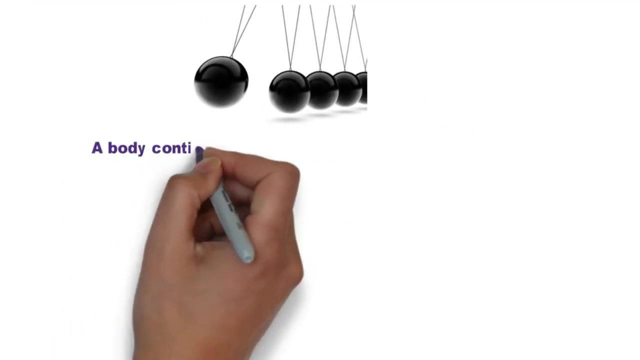 the mass of the Earth is very much greater than the object, and so the gravitational force between them makes objects fall towards the Earth. That is why lead and feather fall at the same rate in a vacuum. Newton's First Law of Motion: A body continues in its state of rest or of uniform motion in a straight line. 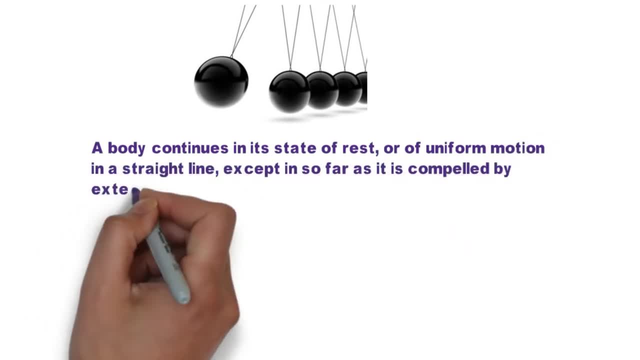 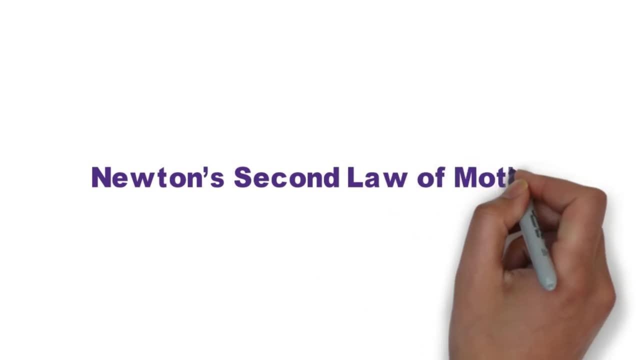 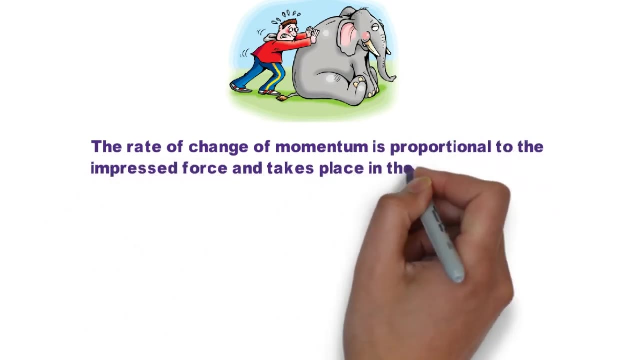 except in so far as it is compelled by external impressed forces to change that state. It is also called Law of Inertia, Newton's Second Law of Motion. The rate of change of momentum is proportional to the impressed force and takes place in the direction of the straight line in which the force acts. 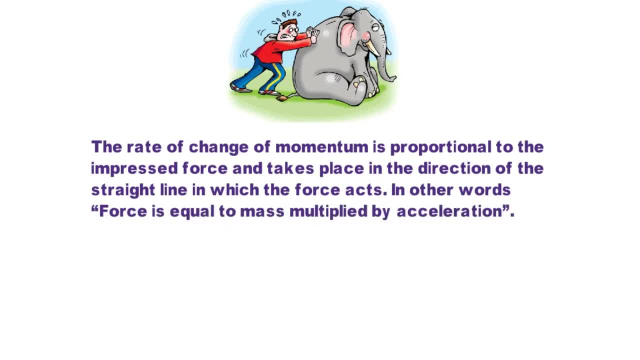 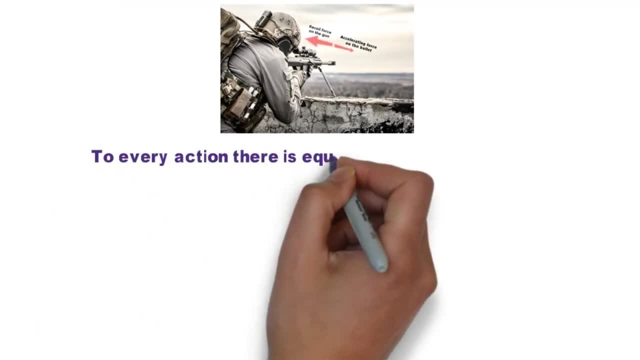 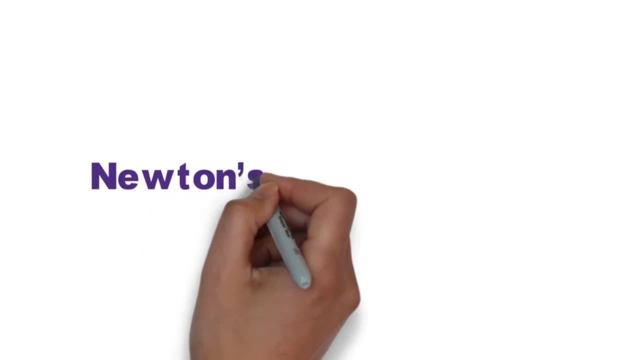 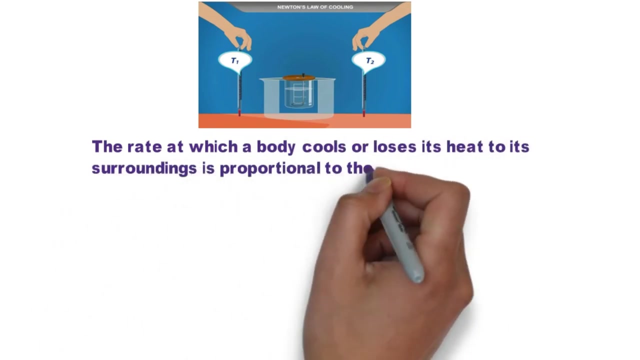 In other words, force is equal to mass multiplied by acceleration. Newton's Third Law of Motion: To every action there is equal and opposite reaction. This is the principle behind the recoil felt on pulling the trigger of a gun. Newton's Law of Cooling: The rate at which a body cools or loses its heat to its surroundings is proportional to the excess of mean temperature of the body over that of the surroundings, provided this temperature excess is not too large. 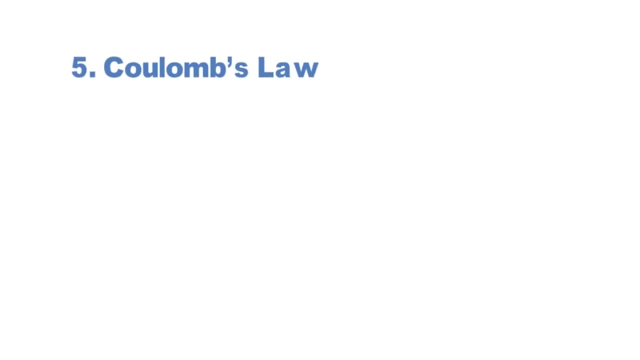 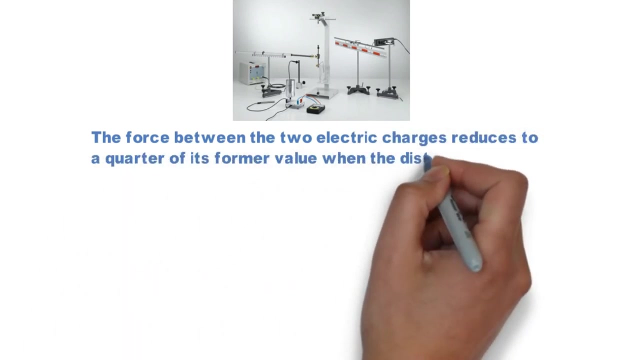 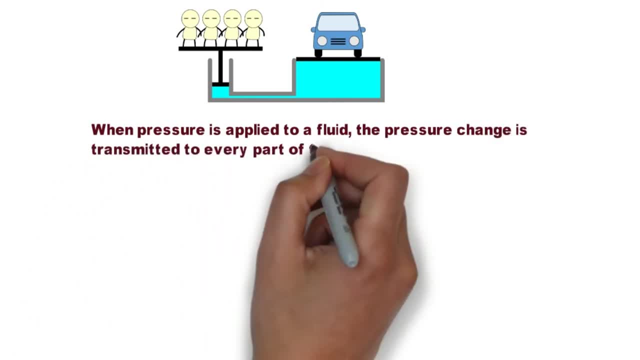 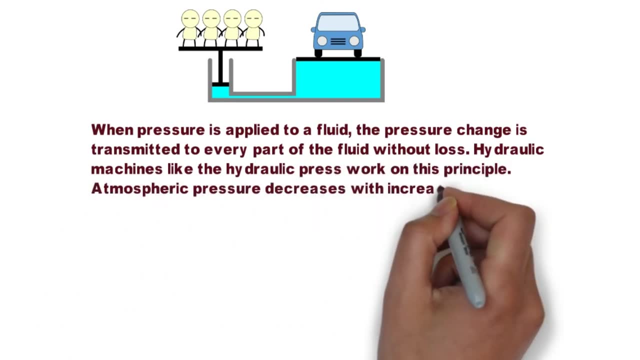 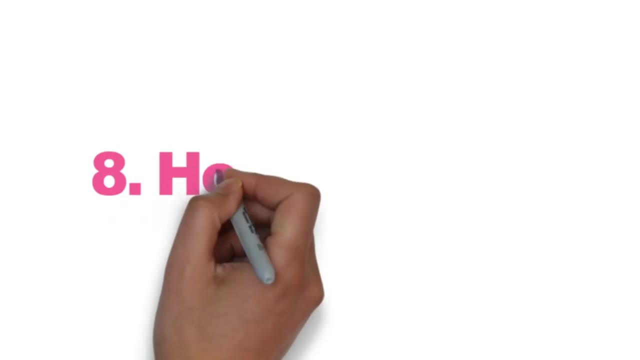 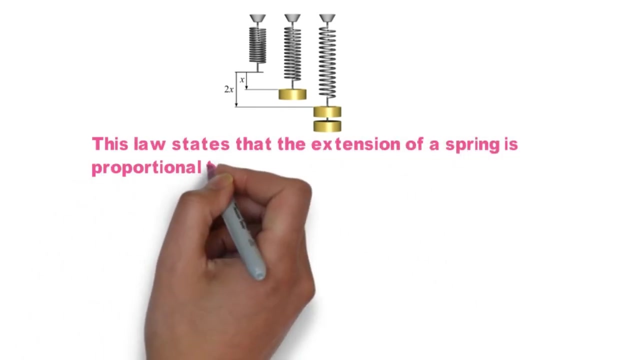 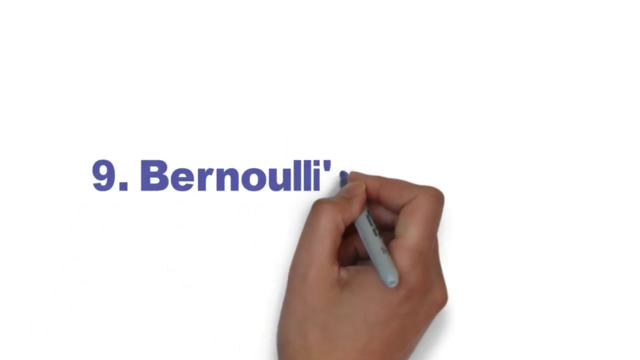 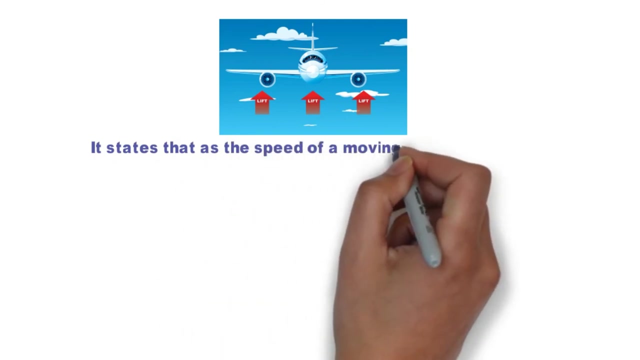 Newton's Third Law of Cooling, The first and second pressures are divided into two. divided into two and divided into two, is, is, is and 9.. Bernoulli's principle: It states that as the speed of a moving fluid, liquid or gas- increases, the pressure within the fluid decreases. 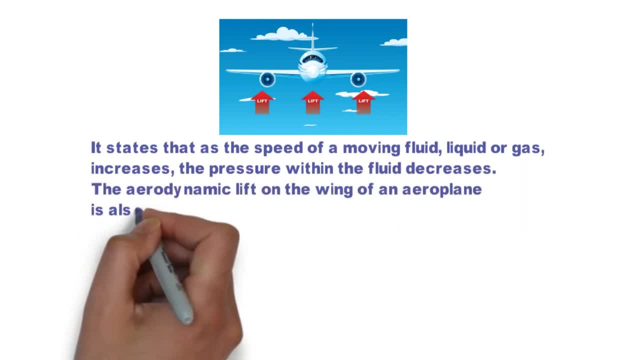 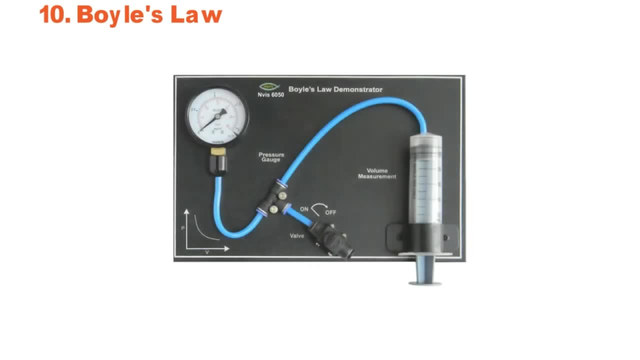 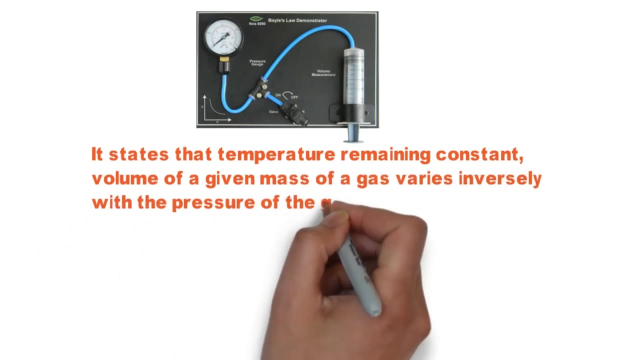 The aerodynamic lift on the wing of an airplane is also explained in part by this principle. 10. Boyle's law: It states that, temperature remaining constant, volume of a given mass of a gas varies inversely with the pressure of the gas. 11. Charles's law: 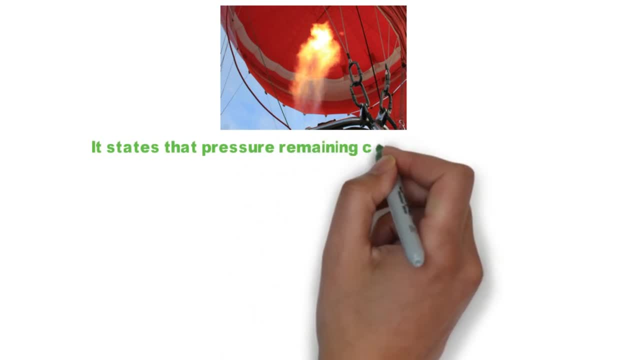 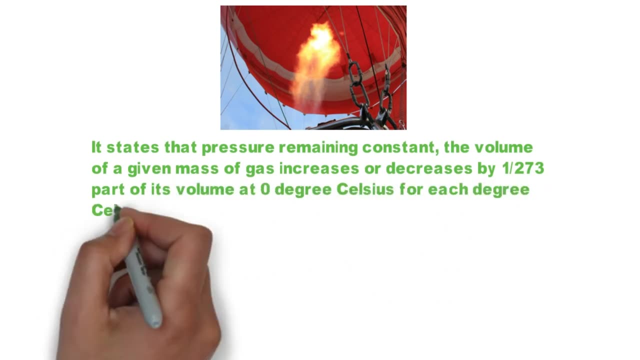 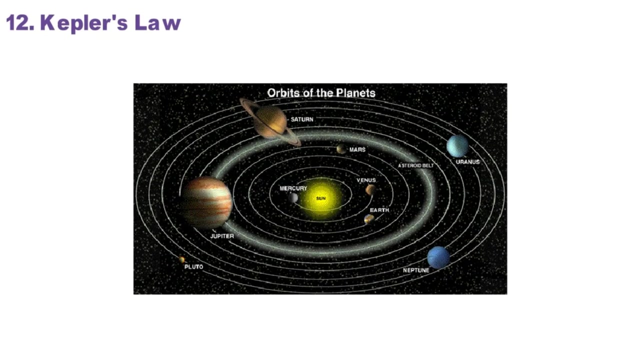 It states that, pressure remaining constant, the volume of a given mass of gas increases or decreases by 1.273 part of its volume at 0°C, for each degree Celsius rise or fall of its temperature. 12. Kepler's law: Each planet revolves round the sun in an elliptical orbit, with the sun at one focus. 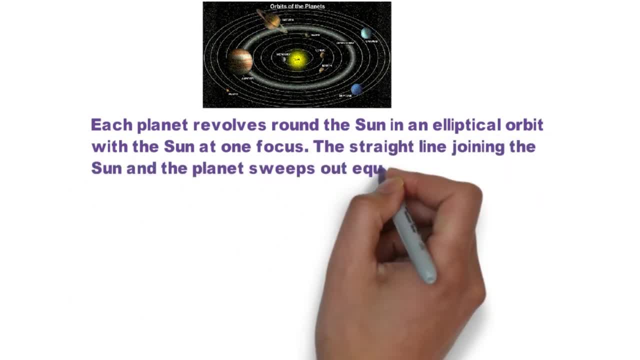 The straight line joining the sun and the earth is called the Kepler's law. The plane of the sun and the planet sweeps out equal areas in equal intervals. The squares of the orbital periods of planets are proportional to the cubes of their mean distance from the sun.